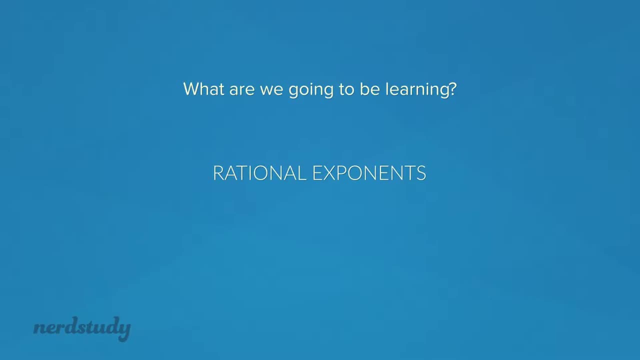 Today we're going to be learning about rational exponents. So far, the exponents that we've been considering were integers, negative numbers, zeros, positive numbers, but we never looked at fractions as exponents. For example, if we have something like 4 to the exponent 1 over 2, what would that be? It's certainly 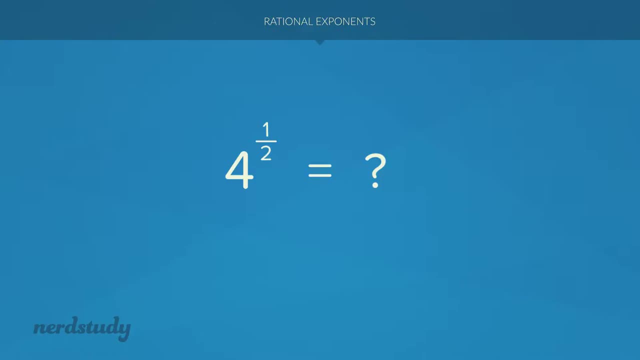 difficult to understand what this would mean, but there is another equivalent form that might help us to understand what this means. Now, this over here is equal to this, So notice how this exponent over here has a numerator of 1 and a denominator of 2.. 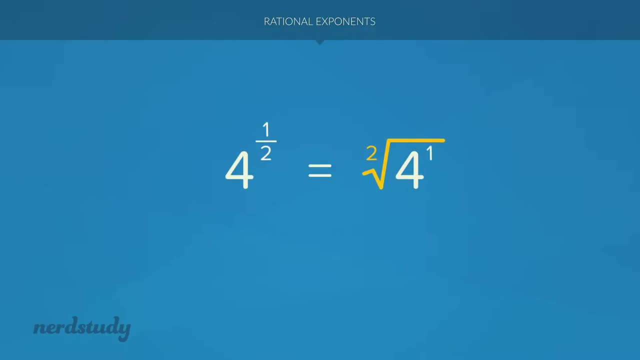 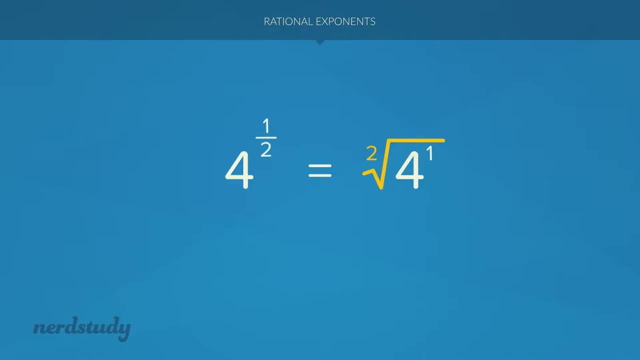 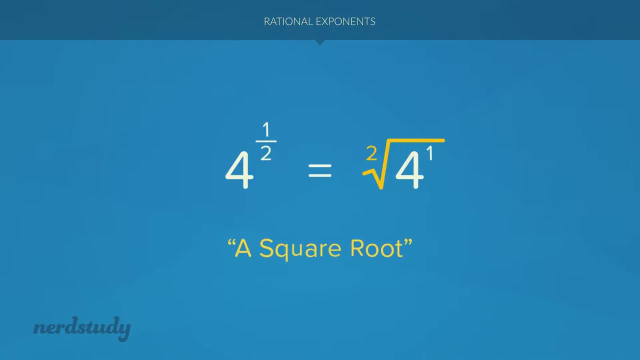 more commonly known as a square root, And since the numerator is 1,, we're looking for the square root of 4 to the exponent 1.. And, of course, the square root of 4 can be further simplified to 2.. Great, So if we had something like 16 to the exponent 1 over 2, then this would be. 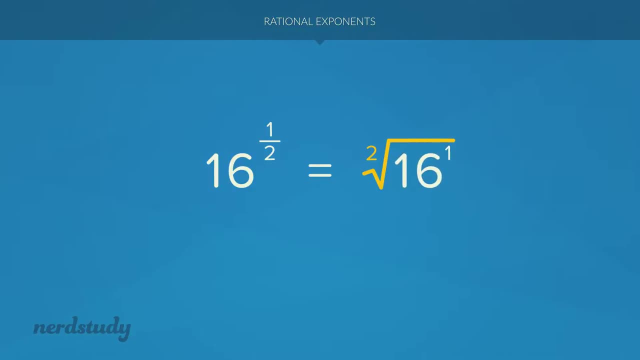 the square root of 16 to the exponent 1.. Of course, that simplifies down to 4.. And we can say this in a general sense. Notice here what is happening to b and what is happening to a. Now, with that in mind, let's try another. 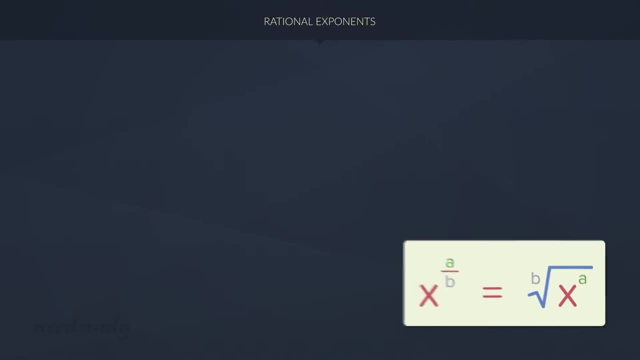 example where we specifically try to use this general formula, And you'll notice that it's actually really easy to do. So. if we had something like 32 to the exponent 3 over 2, that would just be the square root of 32 to the exponent 3.. If it helps you to understand, 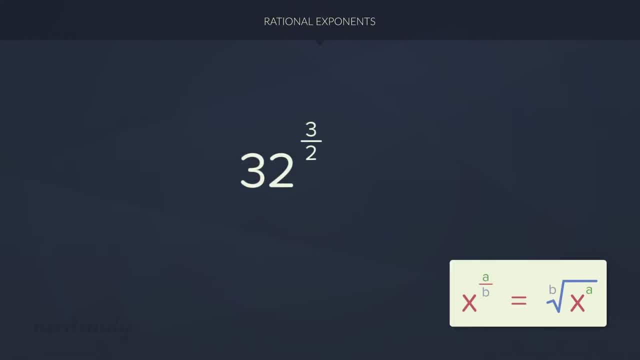 exponents better. another way to do this would have been to see this 3 over 2 as the same thing as 3 times 1 over 2.. After all, 3 is equal to 3 over 1. And when you multiply the numerators, 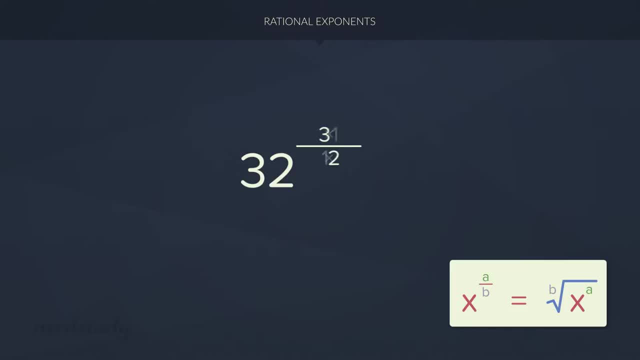 and the denominators, you would end up at 3 over 2.. Now, if you decide to see the exponent as 3 times 1 over 2, then you might also be able to see that this is essentially a power of a power situation. 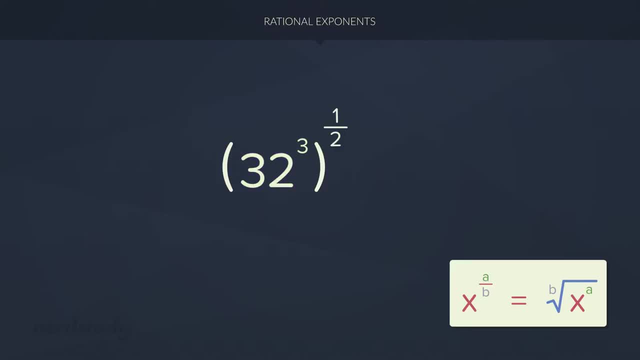 where you have 32 to the exponent 3.. Bracket it to the exponent 1 over 2.. And now, of course, you see the similarities between this example and our very first example, where we did 4 to the exponent 1 over 2.. 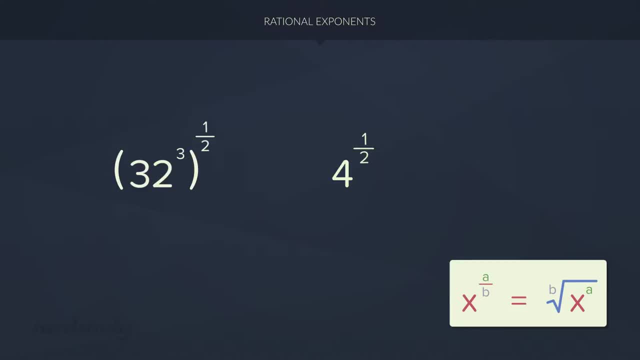 Remember that when we raised 4 to the exponent of 1 over 2, it was the same thing as simply taking the square root of 4.. Similarly, if we're raising 32 to the exponent, 3 to the exponent of 1, over 2, it's going to be equal to t, minus 32 to the exponent 3 over 2.. So we're just going to take 4 to the exponent of 1 over 2.. Now, on the other hand, what we're doing is we're taking 32 to the. 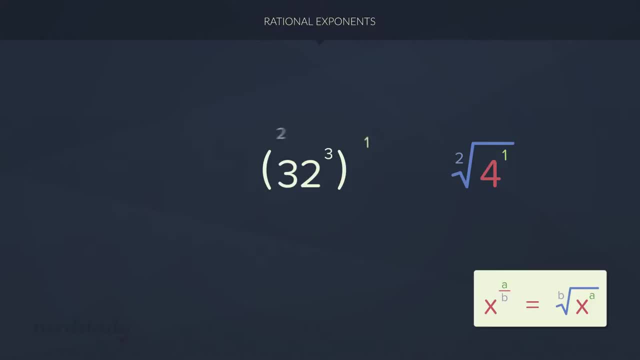 then that would be the same as taking the square root of this entire power right here. Awesome, So let's just do one last question. Let's make this a little bit more difficult, but don't let that fool you. This isn't actually as 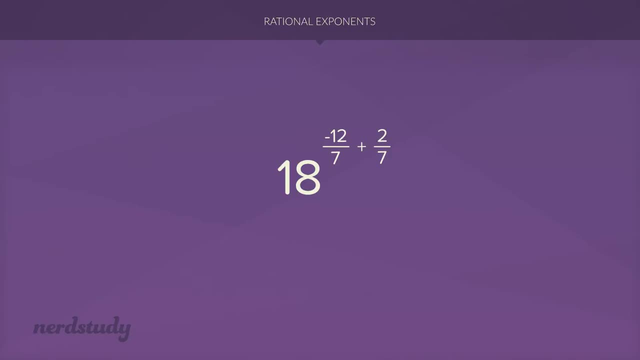 difficult as it might seem. So we have something like this: We see some fractions in the exponents. Well, first, all we have to do is deal with the operators Negative: 12 over 7 plus 2 over 7, well, that's pretty simple. That's just. 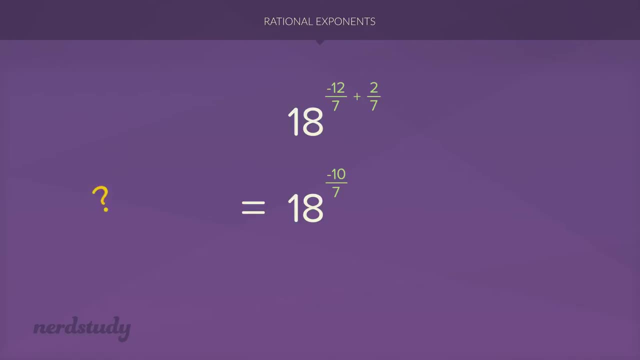 going to be negative 10 over 7.. Now the question is: what do we do from here? Well, we have already learned what to do with negative exponents. 18 to the exponent negative 10 over 7 is going to be the exact same thing as one over 18 to the. 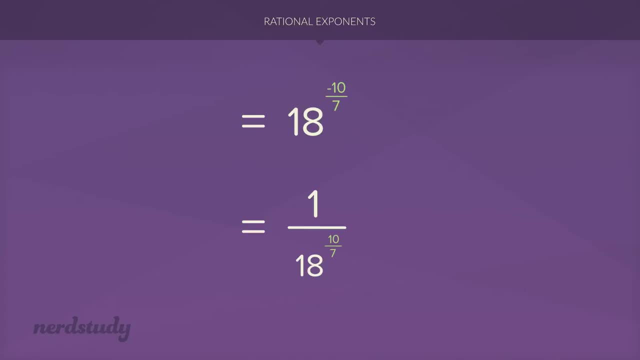 exponent 10 over 7.. Remember, we can just do one over and take that entire power out. It then gives out a negative 10 and there's 7 fractions about there. Now there is well. remember, we can just do one over and take that entire power.